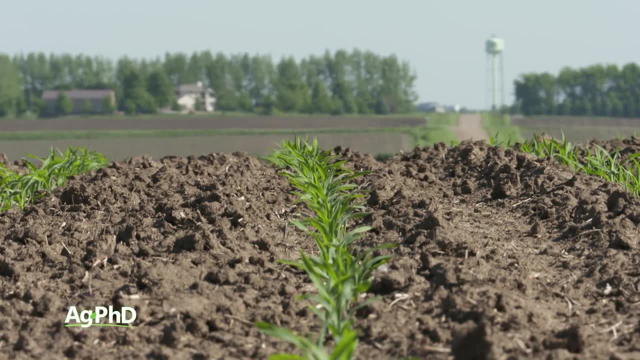 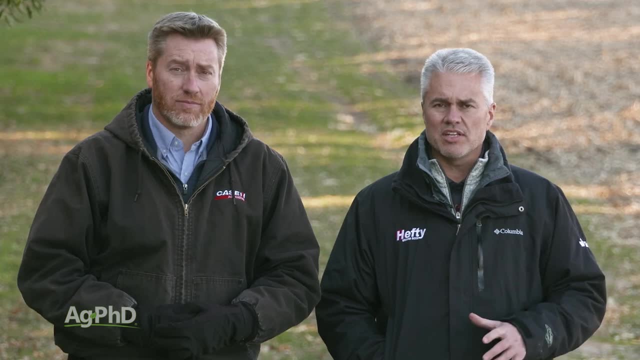 single day. So about I don't know- six, seven years ago, something like that, we talked to South Dakota State University because they wanted to have a weather station just in our region and we said: you know what we'd be willing to sponsor. 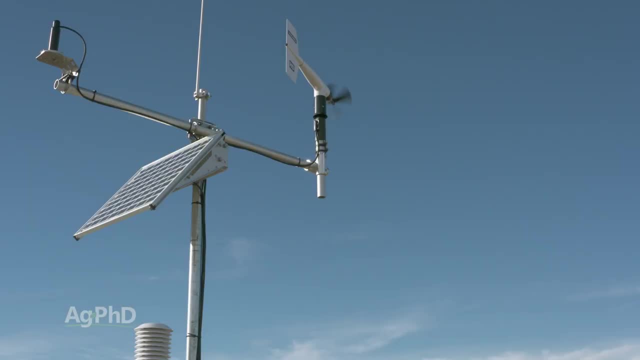 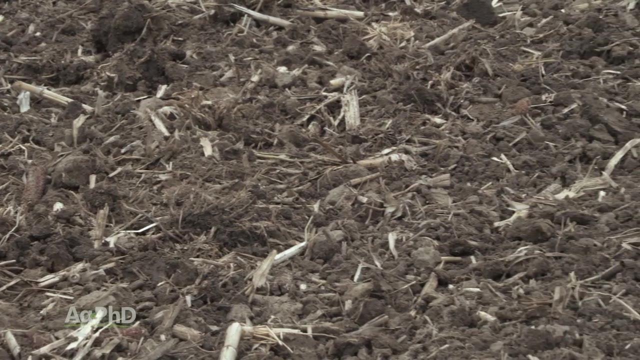 that put it right on our farm. that'd be great. it'd be super interesting and a learning experience. Well, one of the things I learned the most about was soil temperature, because I just assumed you know what a soil temperature can vary- two or three degrees if we're 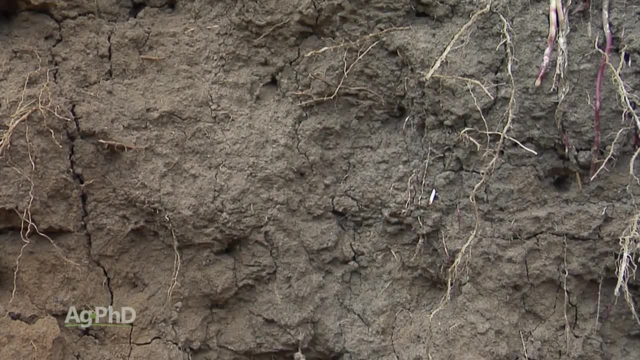 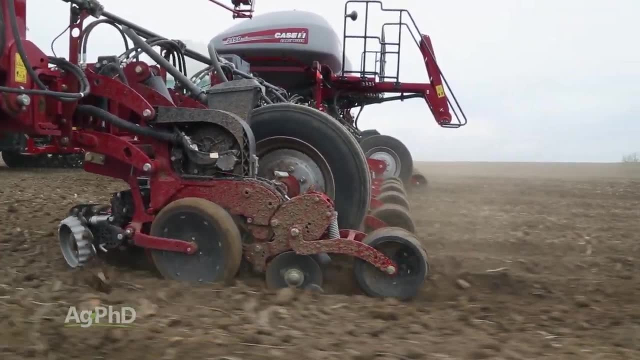 looking at four inches deep down in the soil, because I mean every year we would look at when we're going to plant what's the soil temperature, what's the temperature and all that kind of thing. Well, with this weather station that they put up, it would measure. 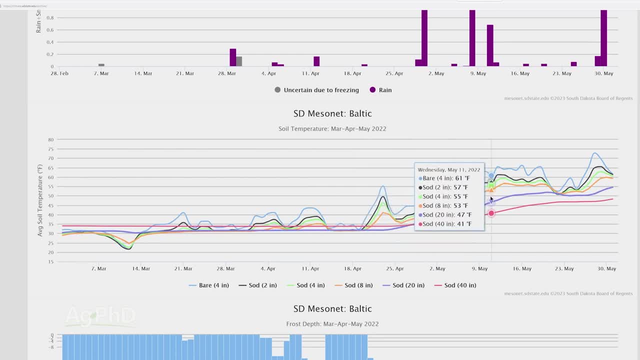 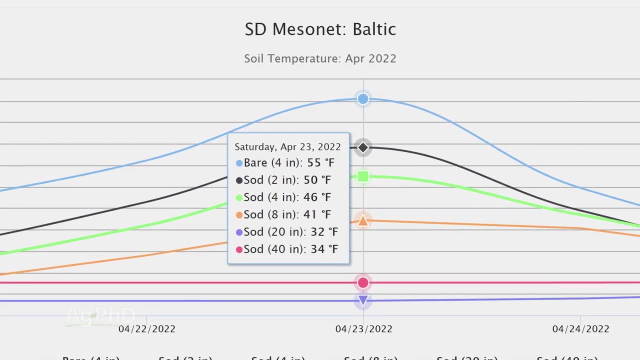 temperature, soil temperature: four inches deep every five minutes. And so now we have all kinds of data from the last quite a few years and it is shocking to me how much, just in a single day, that soil temp can vary, And I'm pretty sure Brian was just watching that. 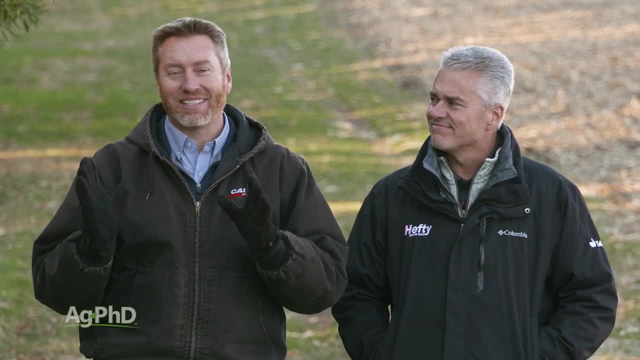 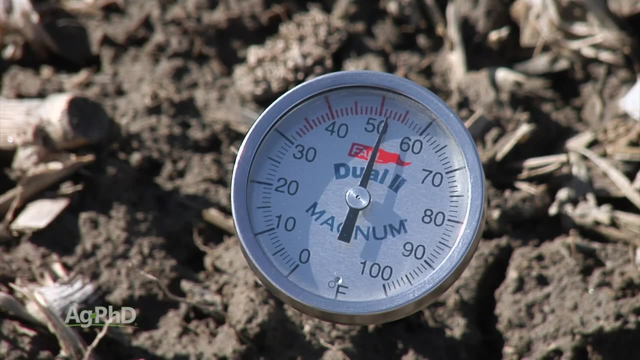 gauge every five minutes through the day to see what it went, because in the spring we are watching it and we are thinking: well, everybody says we need to plant at fifty-degree soil temperature and it's not going to happen. It was really amazing for me to see. 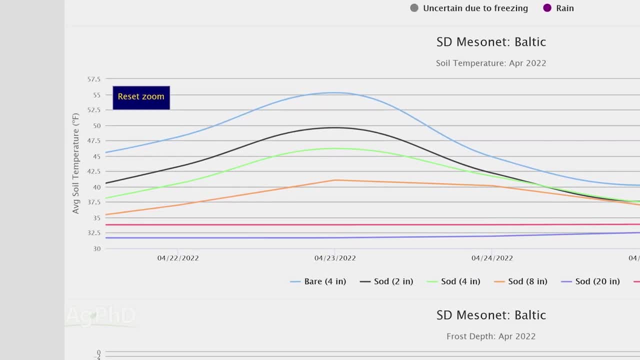 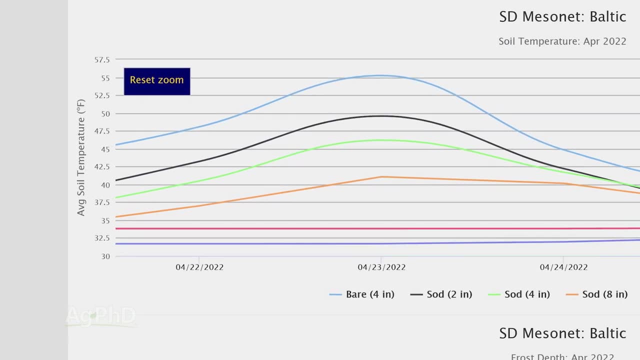 wow, that soil temperature varies a lot during the day and even days that start out kind of cool could be fifty degrees later, or they could start out warm and be cold later. That's the whole thing. So when I'm talking to farmers that say, well, I have to plant when the soil 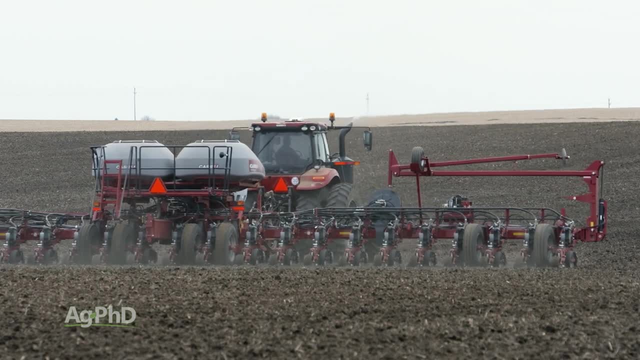 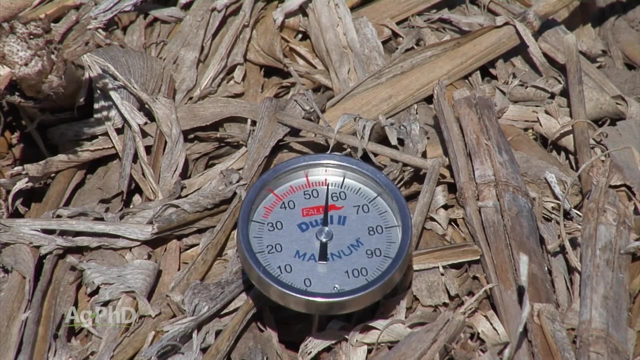 temp's fifty. I'm like: well, you know what, on my farm it was thirty-six, but it was also fifty-six. They're like what? No, Yes, we've had many, many days in the spring where the soil temp will vary twenty degrees in a 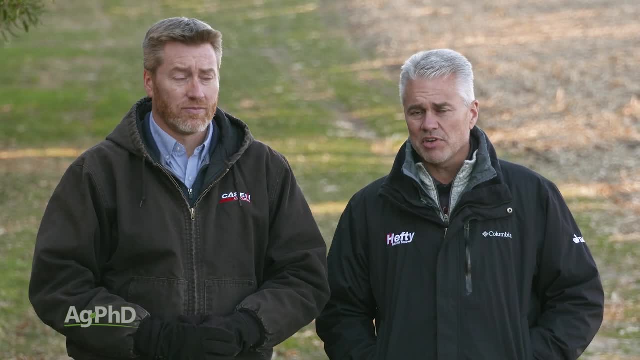 single day, and that's in the spring, And that's the whole thing. Now, when we get into the summer, could it vary even more than that? Sure it could. So when you start thinking about, alright, what's the soil? 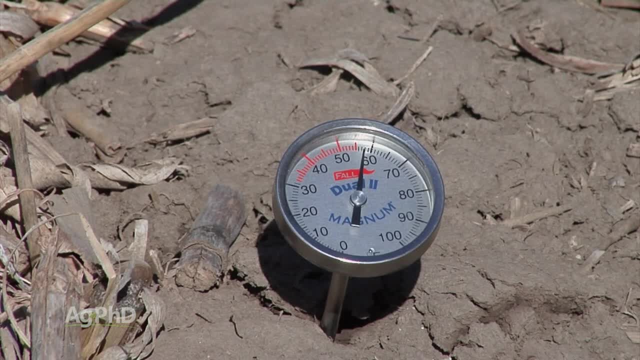 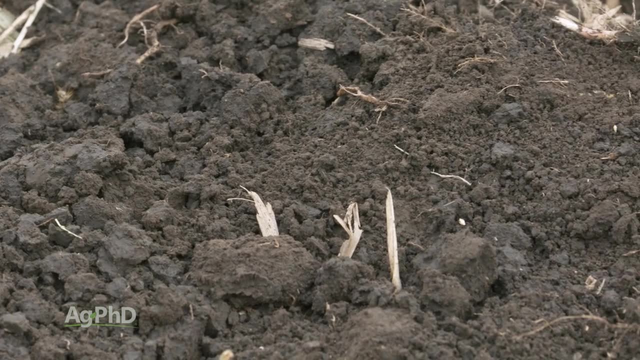 temperature. what's that ideal soil temp that I want to plant at? just understand that it's going to vary a lot during the day. and that's at four inches deep and we have pretty heavy soil And I could see it if I had. 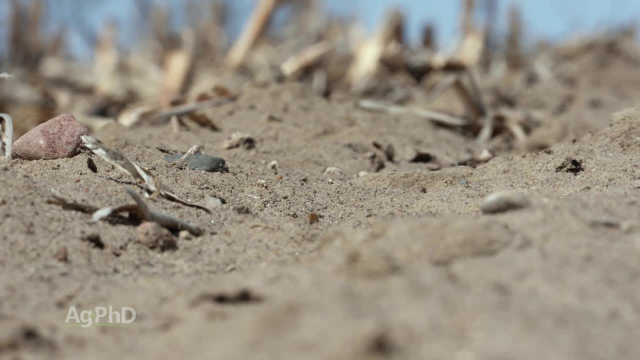 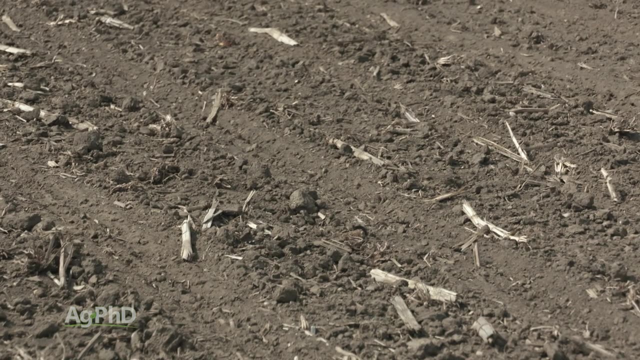 lighter soil that it would vary more. I can also say this: if your soil is drier, it will vary more than if your soil is wetter. So just something to keep in mind Now in the middle of the growing season here.